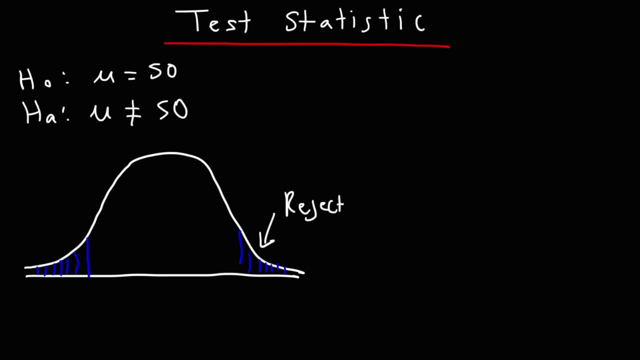 The area shaded in blue is known as the rejection region. The area that is not shaded is the fail-to-reject region. Now the z-values that separate these two regions. these are the critical values. Now, let's say, if we're dealing with a 95% confidence level, You could use the standard z-tail. 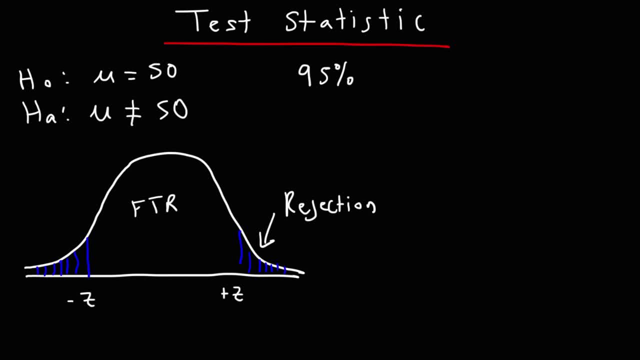 table to get the z-values. So, at a 95% confidence level, the critical values will be 1.96 on both sides. Now, in order to know whether you should accept or reject the null hypothesis, you need to get another z-value, a calculated z-value, and compare it to your critical value. Let's call. 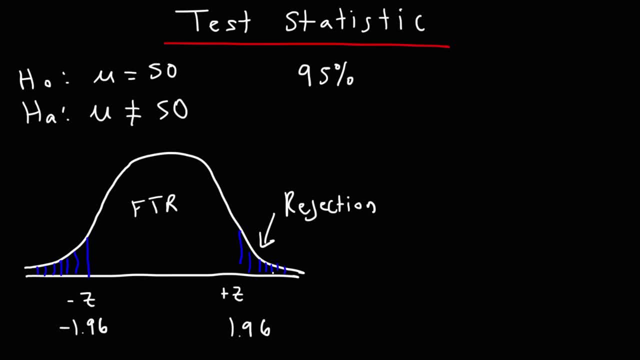 that calculated z-value zc. Let's say, if zc is the z-value of zc, then the z-value of zc is the z-value of zc. If zc is to the right of z, then that means that you should reject the null hypothesis. 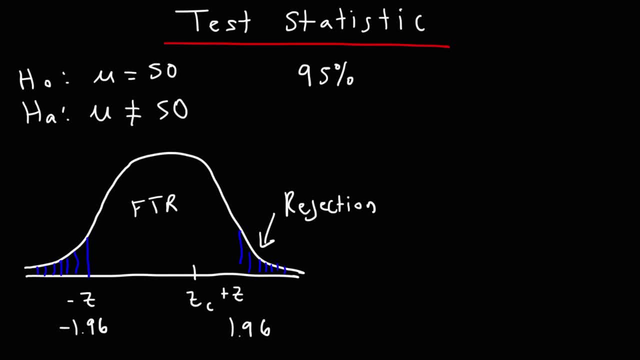 If zc is to the left of z, that is, if it's in the fail-to-reject region, you shouldn't reject the null hypothesis, You should keep it. So now let's talk about how we can calculate zc. So this is: 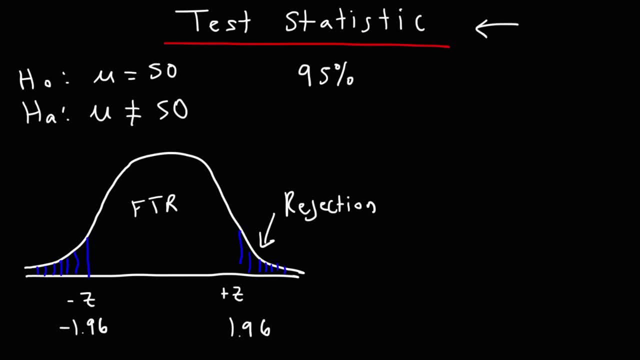 known as the test statistic. So first let's talk about if we have a population mean versus a population proportion. Now, sometimes you may need to use the t-distribution, Other times we need to use the normal distribution and get the z-value. So let's say that the sample size is less than 30 and that the population standard 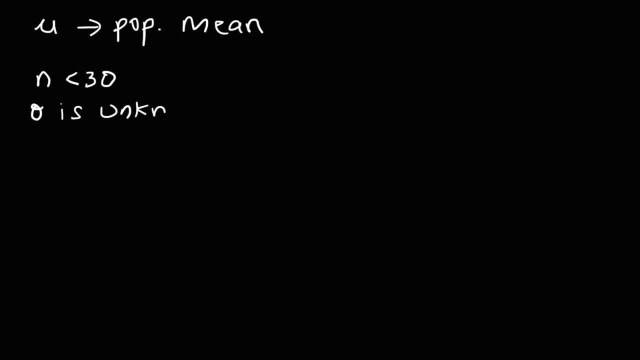 deviation is unknown. So if these two conditions are met, in that case we need to use the t-distribution. So our t-value is going to be the sample mean minus the population mean divided by the sample standard deviation over the square root of n, where n is the sample size. Now let's say that n is less than 30,. 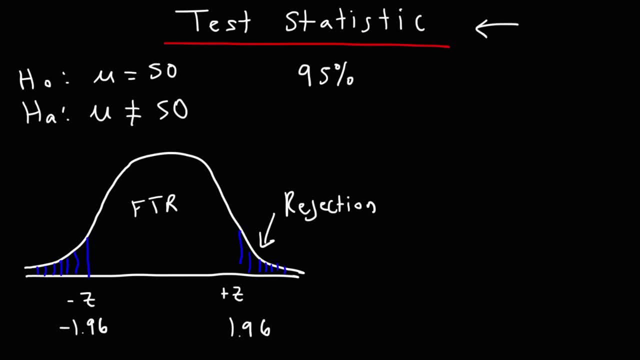 known as the test statistic. So first let's talk about if we have a population mean versus a population proportion. Now, sometimes you may need to use the t-distribution, Other times we need to use the normal distribution and get the z-value. So let's say that the sample size is less than 30 and that the population standard 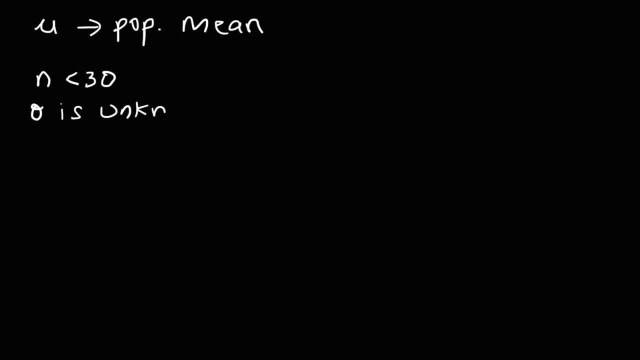 deviation is unknown. So if these two conditions are met, in that case we need to use the t-distribution. So our t-value is going to be the sample mean minus the population mean divided by the sample standard deviation over the square root of n, where n is the sample size. Now let's say that n is less than 30,. 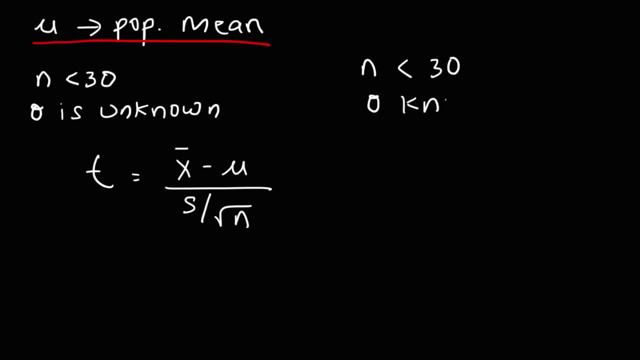 but we know the population standard deviation. In this case we could use a normal distribution. So we're going to calculate the z-value. So our calculated z-value is going to be the sample mean minus the population mean divided by the standard deviation, that is, the population standard deviation over the square root of n. 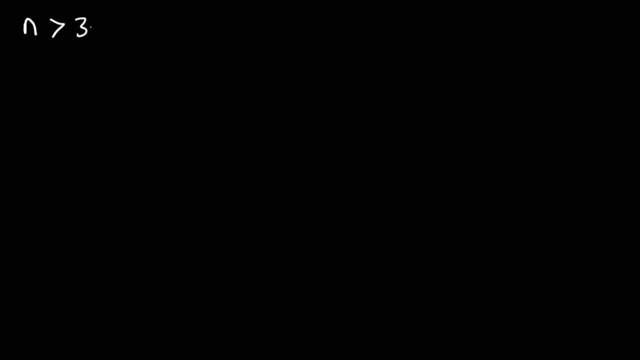 So, for example, we can layer it to the right and divide that by 2 and we get thisantine function. Now let's say that n is greater than 30 and the population standard deviation is unknown Because the sample size is large. 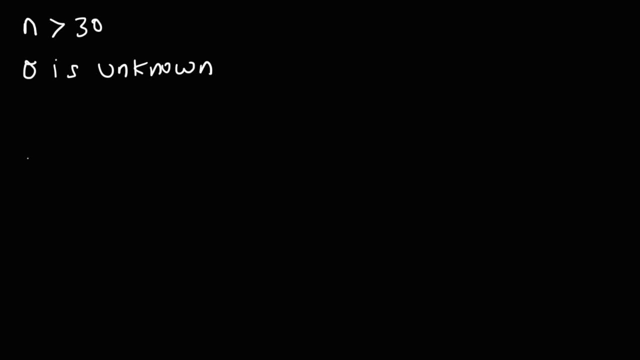 the distribution will be similar to a normal distribution. So once again we can calculate the z-value. So it's going to be the sample mean minus the population mean divided by the sample stand deviation, which is now the same as the population standard deviation. 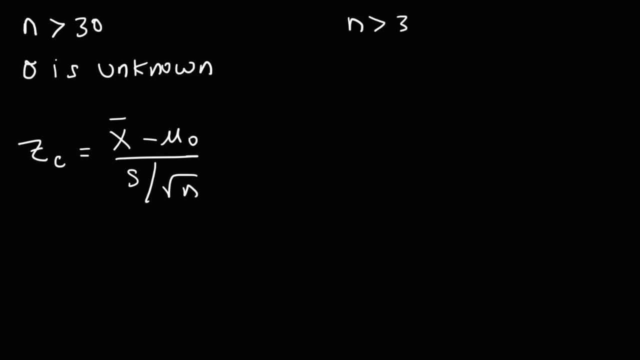 deviation over the square root of n. now, if n is large and if we know the population standard deviation, everything is going to be the same. instead of using s, we're going to use Sigma. so those are the formulas in which we can calculate the Z value or our T value and compare it to the critical value in order to 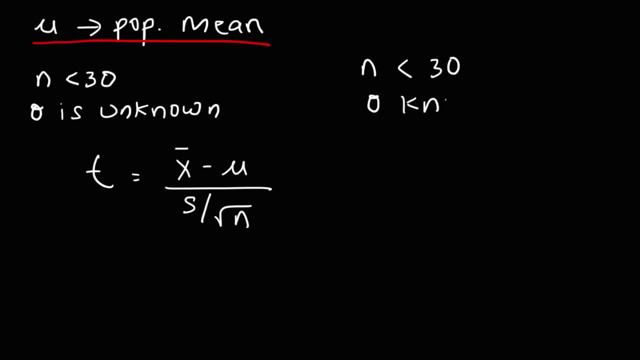 but we know the population standard deviation. In this case we could use a normal distribution. So we're going to calculate the z-value. So our calculated z-value is going to be the sample mean minus the population mean divided by the standard deviation, that is, the population standard deviation over the square root of n. 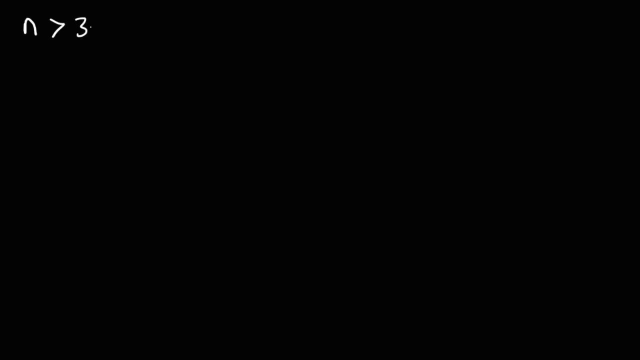 Now let's say that n is greater than 30, and the population standard deviation is unknown. Because the sample size is large, the distribution will be similar to a normal distribution. So once again we can calculate the z-value. So it's going to be the sample mean minus the population mean divided by 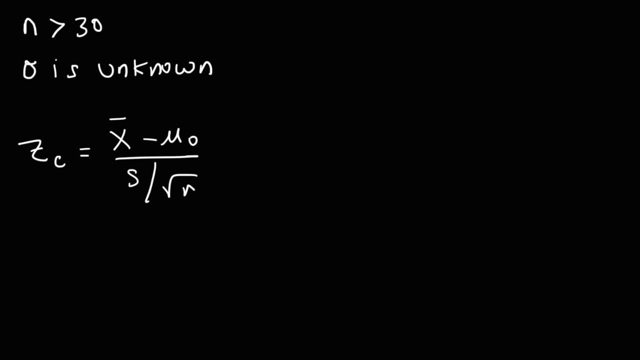 the sample standard deviation over the square root of n. Now, if n is large and if we know the population standard deviation, everything is going to be the same. instead of using s, we're going to use sigma. So those are the formulas in which we can calculate the z value or our t value and compare. 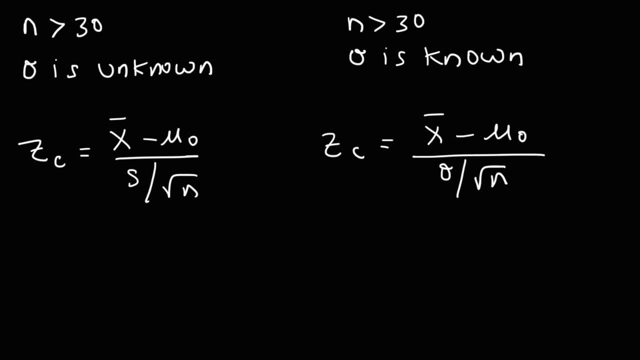 it to the critical value in order to determine whether we should reject the null hypothesis or if we should not reject it. So this is when you have, when you're dealing with the population mean Now, sometimes you can be dealing with the population proportion, and so that's going to be p. 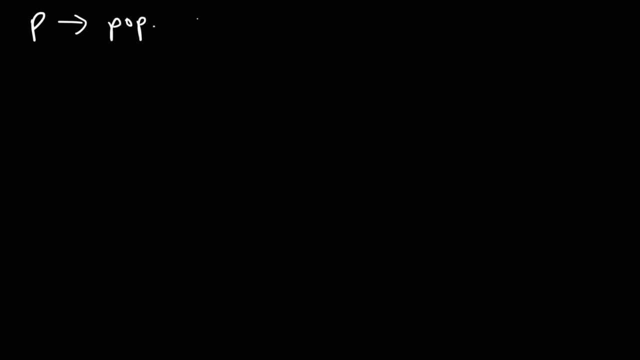 instead of mu. In this case, we're going to use a different formula to calculate the z value. So we're going to use a different formula to calculate the z value- z- and so the formula is it's going to be the sample proportion minus the population. 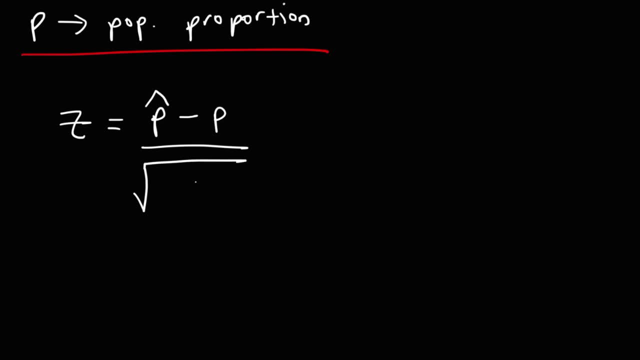 proportion divided by the square root of pq over n. Now n is still inside the square root. q is 1 minus p, so just keep that in mind. So that's the formula we need to use if we're dealing with a proportion. That's how we can get our calculated z value. 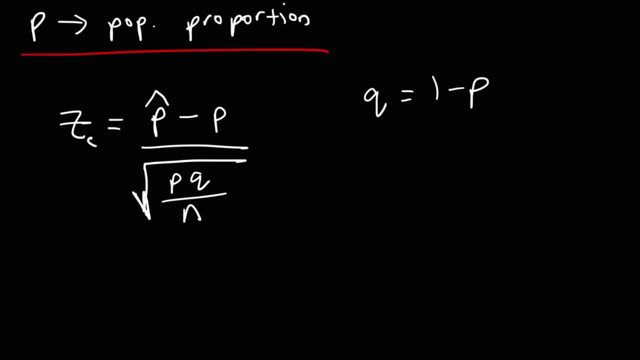 So those are the test statistics that we need to be using when solving problems associated with hypothesis testing.